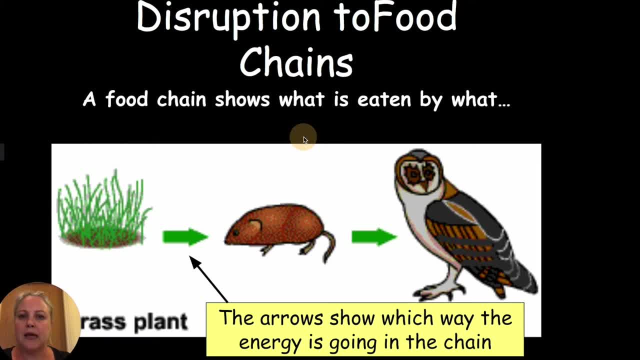 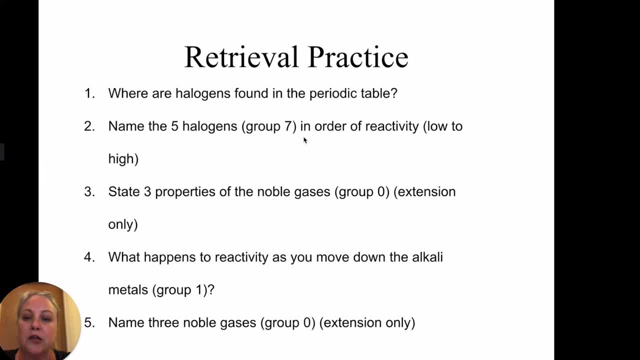 following along on the worksheet. the first thing I'm going to ask you to do is I want you to pause the video and have a go at these five retrieval practice questions based on the topic we did previously to this one. So, pause the video, have a little go at them, and I know you find them tough. 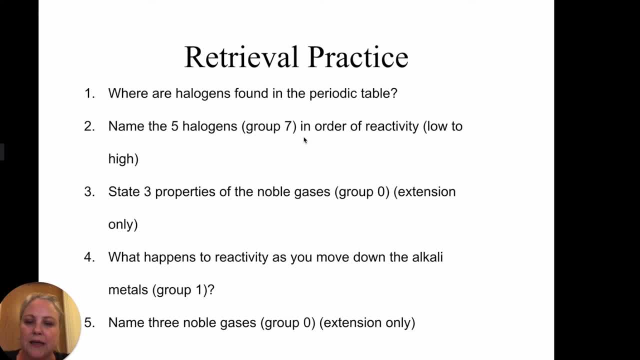 but that's why we need to do them, to get that memory coming back. Okay, so keep making sure that we can find all that knowledge inside our brain. So pause the video, have a go at these questions. they're all going to help you. So I want you to pause the video and have a go at these five. 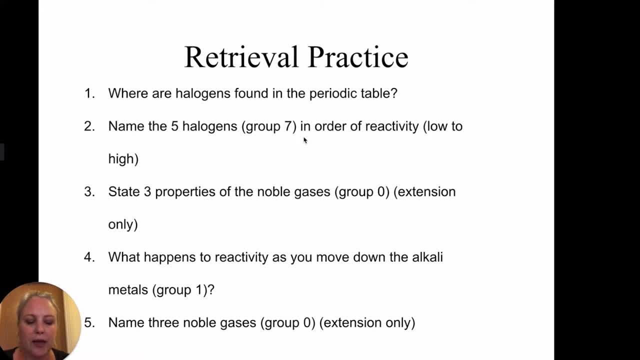 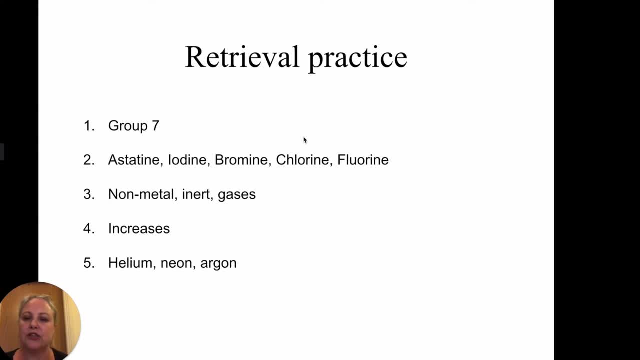 are on the worksheet attached. Okay, so hopefully you had a go. if you didn't make sure, you pause it. now. have a go, Okay, and here are the answers, so you can have a little check against them and go back, maybe rewind the video if you need to. Now I want you to put the following things into a food: 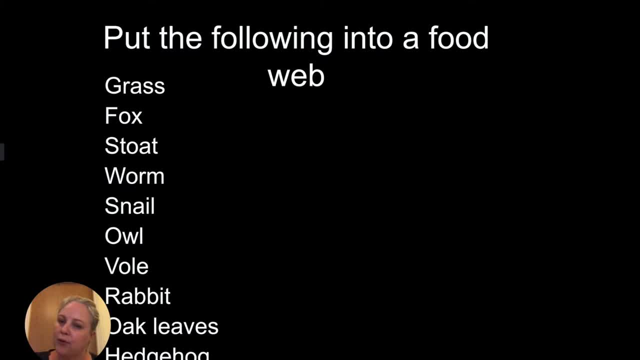 web. Okay, grass fox, stoat, worm, snail owl, vole, rabbit, oak leaf hedgehog. So I want you to pause the video. have a go and put them into a food web. Now. food web will be a bit messy, so you. 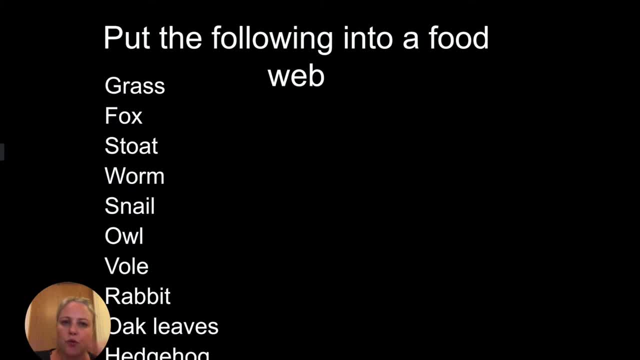 can put it into a food web. So you can put it in a food web. Now, you can put it into a food web. So I suggest you put those names all over your paper and then start drawing the arrows. Remember clearly what the arrows mean. which ways do they point? Okay, so take your time and think about. 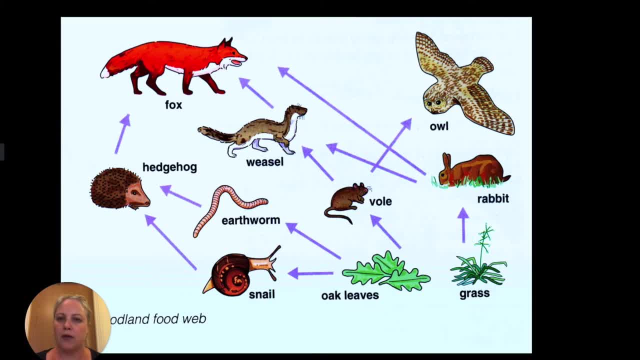 that. So pause the video, have a go. Okay, so you might be coming up with something like this. Notice that which ways the arrows go. The arrows show the flow of energy, So the vole gains energy from eating the oak leaves, So the arrow goes to the vole. The energy goes to the vine, So the 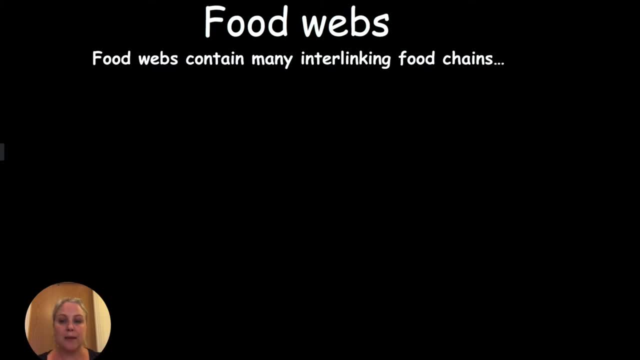 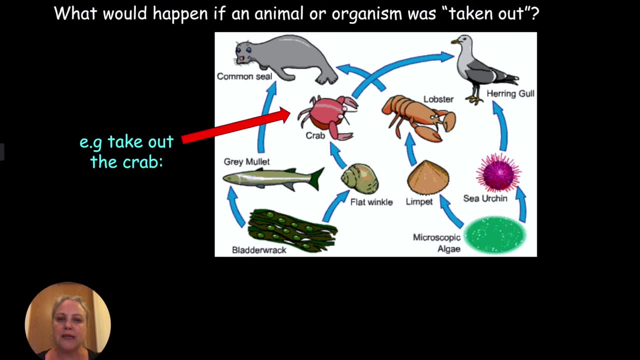 all. so food webs contain many interlinking food chains, so here's another food web for you to have a look at. i'm going to look at this in a bit more detail. okay, so if we take out the crab, what do you think will happen? okay, so it's on the worksheet. i want you to write down the answer. i want you to. 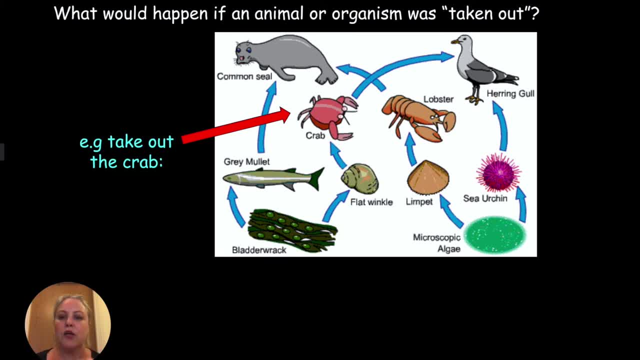 pause the video. what do you think will happen? so if we take out the crab, you need to look at what eats the crab, what's eaten by the crab. what will happen? okay, so think carefully. so if you're still a bit stuck, here's two starter sentences. so the flat winkles would not get eaten, so their